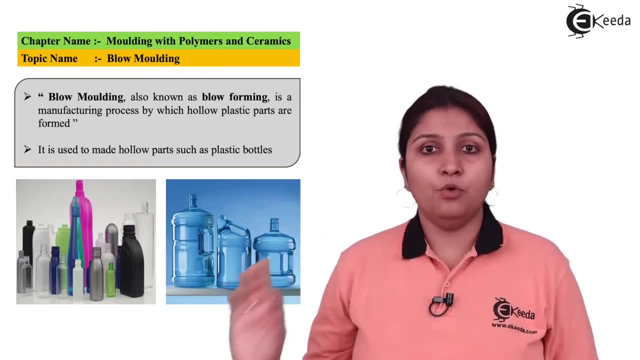 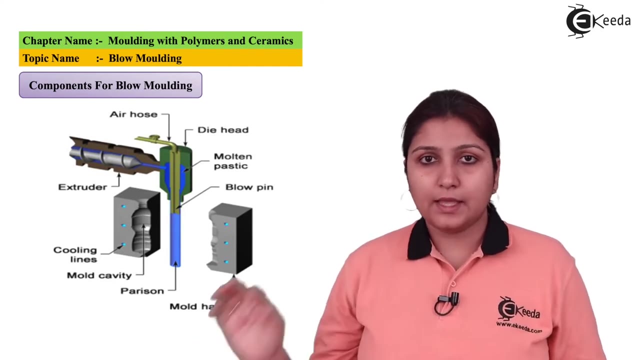 canes, etc. So these are example of blow molding process. Air is blown inside your plastic so that it inflates and form the desired shape which is required. So in this diagram you can see there is an extruder which supplies air to your parasol. What is parasol? It is nothing but a plastic. 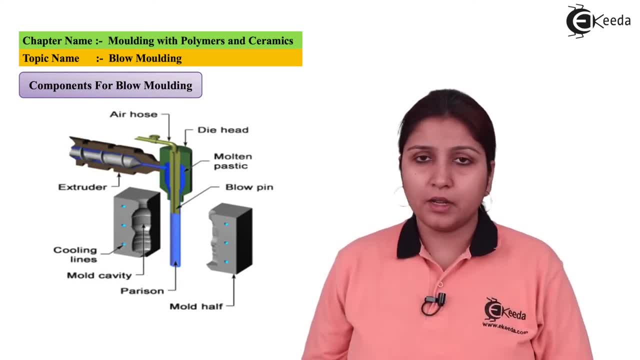 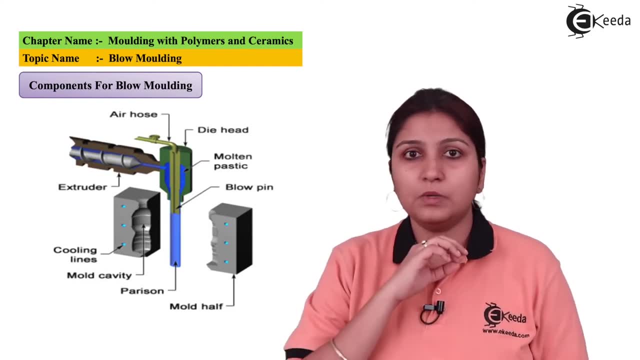 object which is made through different heating and melting processes, but it is hollow from inside, so air is blown inside that parasol, like blowing a balloon. Balloon is being blown by air. The structure of outside balloon is a parasol and you can see there are two dies on right and left of a parasol. 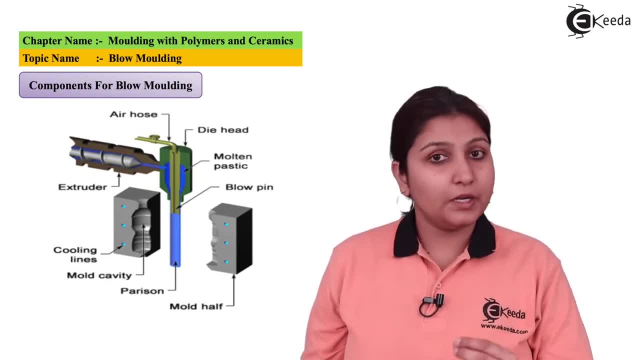 So when you blow a balloon, you can see that there is an extruder which supplies air to your parasol. If your parasol is blown which is a bit heated, it reaches your die cavity, gets its shape and it is. hold it at that position and then, when the die part is removed, your exact shape can be achieved. 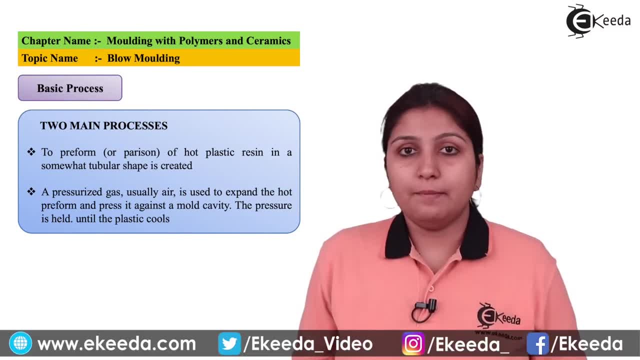 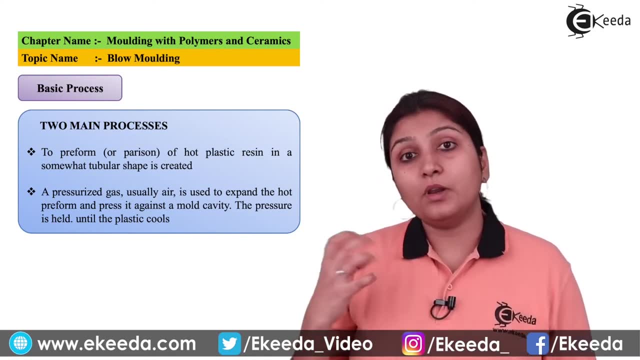 So in blow molding, these two steps are very important. Number one is heated parasol. If your parasol is not heated properly, it won't get blown. So if more heating is provided, it can melt, and if less heating is provided, blowing cannot be done. So educate or opt out of your parasol. 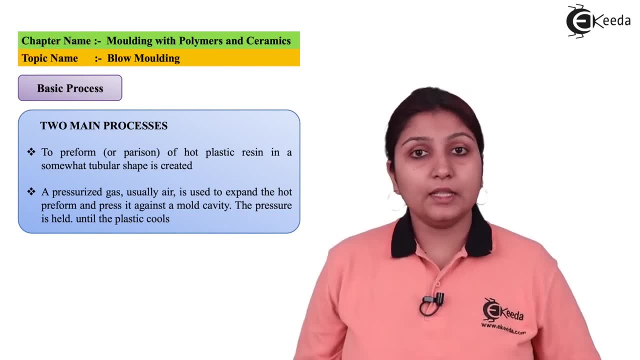 if your parasol has a pore and floor, since it will not remain like a normal parasol. And the second step is you need pressurised air so that the parasol can inflate easily and reach your die cavity. So, in this process, what you are going to do, you are going to keep your die close to each other. 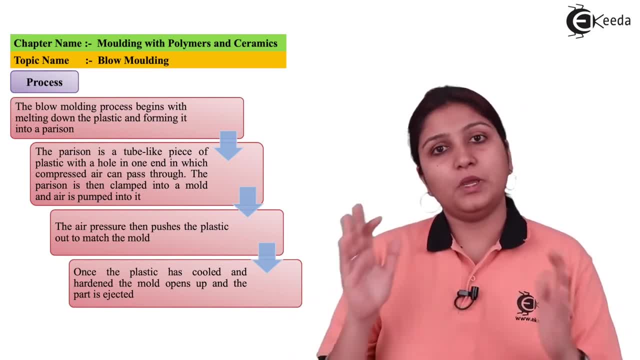 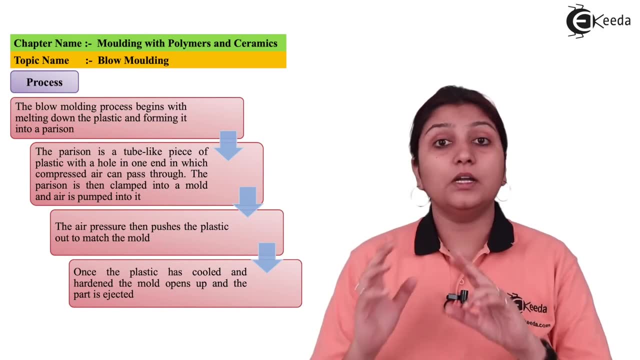 Like. it should not be far away so that parasol cannot reach there. It should be close enough to get the shape of your required object. So let's say, i'll give you an example of a bottle. it has a certain shape, but the heated 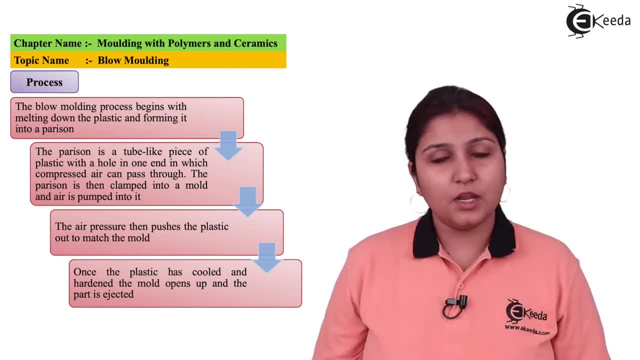 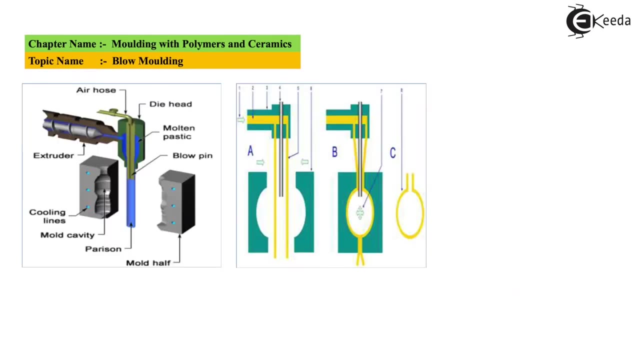 parison gets air and why it gets the shape? just because of the dye, which are close to each other, like of a certain distance, which are prescribed. so in this way bowl molding process takes place. so in this diagram you can see a, b, c. there are three steps: one, blowing. second, getting the shape.